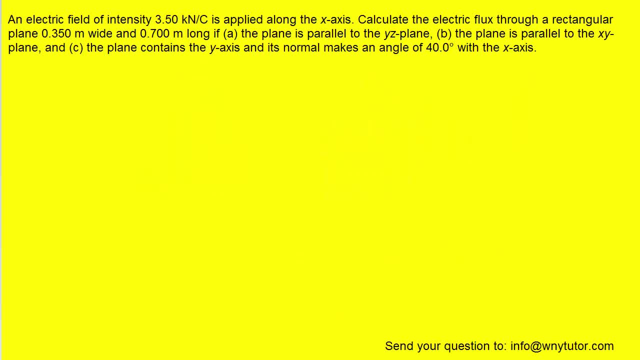 If you haven't done so yet, please pause the video and try to answer the question on your own before listening on. The question is asking us, for each part, to calculate the electric flux, and so why don't we look at the equation for electric flux? And so here we have the Greek letter. 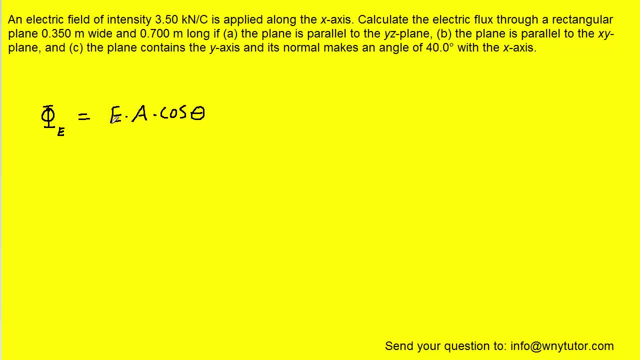 Phi to represent the electric flux, which is equal to the magnitude of the electric field multiplied by the area, multiplied by the cosine of an angle. Now, the angle will be between the electric field direction and the direction of what is called an area vector, and so we'll have 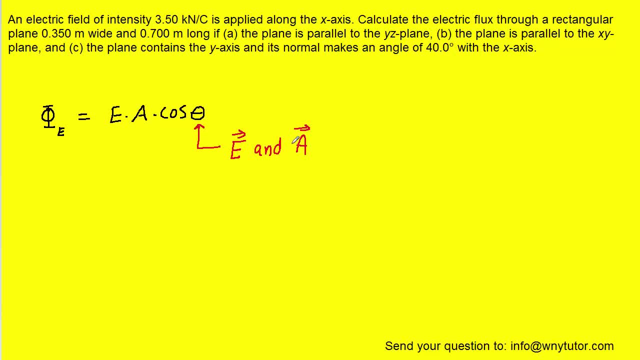 to take a closer look at what these two vectors actually mean. Why don't we actually draw the scenario that's described in Part A? So here we have our traditional y-axis and x-axis, and we have our traditional y-axis and x-axis, and we have our traditional y-axis and x-axis. 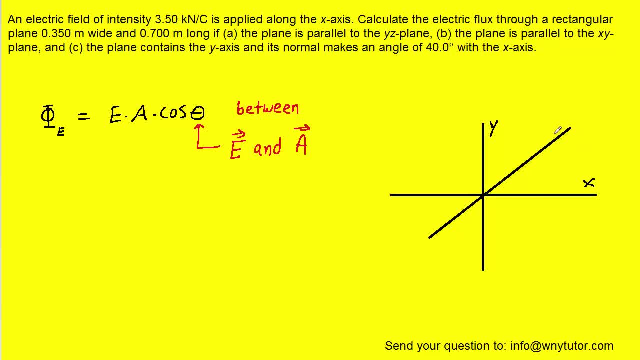 and then we have this third axis that we typically don't deal with in this course, but it does occasionally come up, and that is known as the z-axis, And the question notes that the electric field is applied along the x-axis. so why don't we draw an electric field vector that's pointing in? 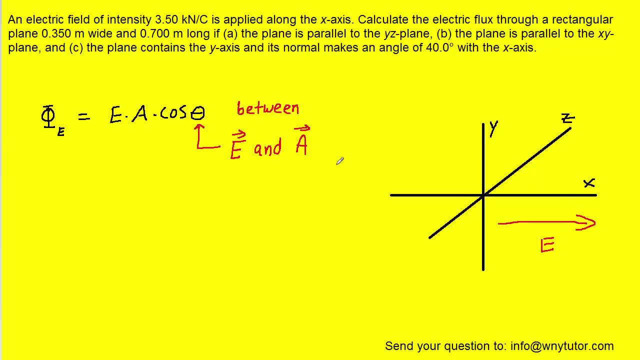 the same direction as the x-axis, And then, for Part A, we're going to attempt to draw a rectangular plane that is parallel to the yz plane, And so the yz plane would be this region right here, and if we were to draw a rectangular plane, 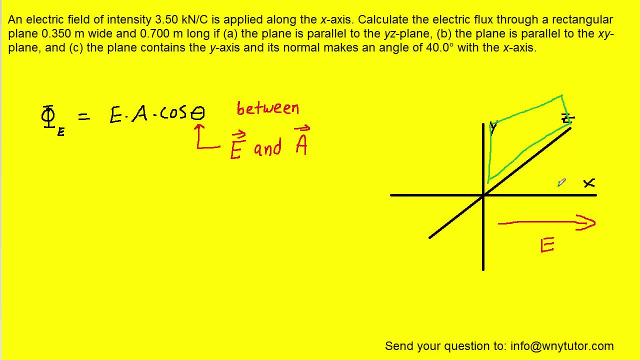 that is parallel to that. we would basically draw another rectangle that is sort of a carbon copy of the one we just drew. It's a little challenging to draw, but hopefully it makes some sense. It actually might even make more sense if we just stick with this original rectangular plane, right. 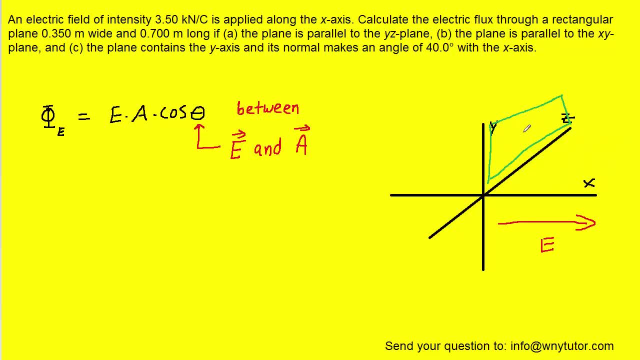 here. So why don't we go ahead and omit this one? And with that rectangular plane we can draw what is known as an area vector, and an area vector will always point perpendicular to the rectangular plane, So we would draw a vector. that's sort of. 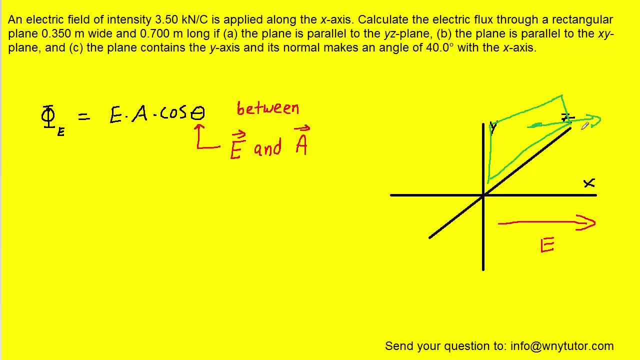 projecting in this manner right here, And what you want to ask yourself is: what is the angle between this area vector and the electric field vector that we had drawn just a moment ago? And hopefully we can see that the angle between these two vectors is actually zero degrees. So for part a, we're going to be plugging in zero degrees, for theta, and we have 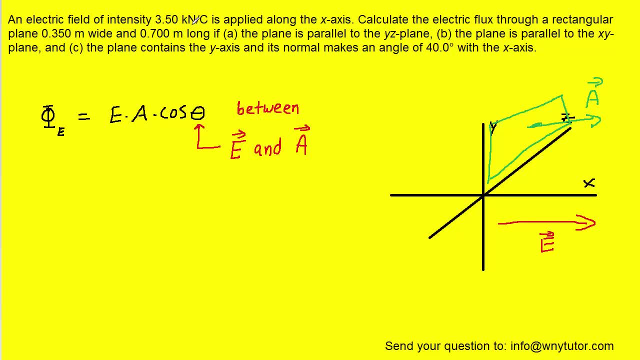 the electric field given to us, Notice it's in kilonewtons per coulomb, So we might want to convert that into newtons per coulomb by multiplying it by a thousand, And then the area- because it's a rectangle- will simply be the length of the rectangle multiplied by its width. And I actually 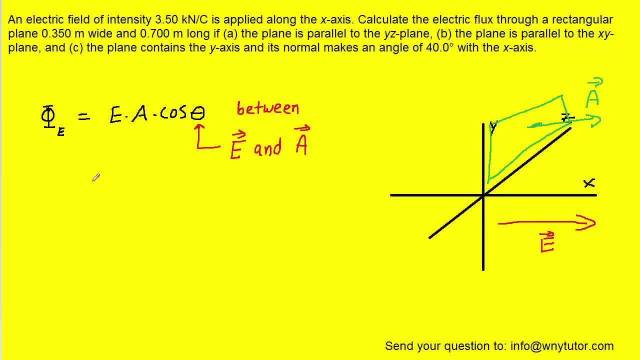 think I just flipped those around. So this is the length and then this is the width. So we'll go ahead and set up the electric flux formula And when you multiply the electric flux formula you'll see that the electric flux formula is in kilonewtons per coulomb. So if you multiply that all out you should get roughly 858.. And then the 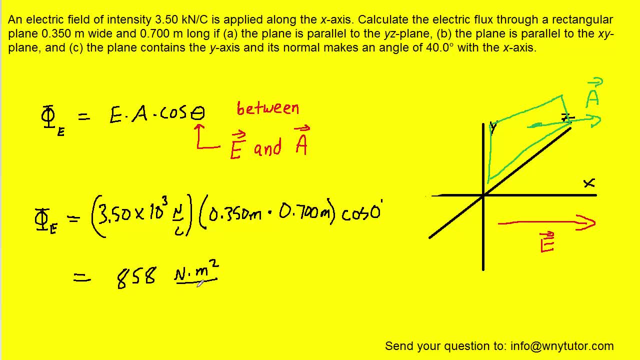 unit here is going to be newtons times meters squared per coulomb. Once again, note that we converted the electric field strength into newtons per coulomb by multiplying it by 10 to the power of 3.. So this would be the final answer to part a. So now on to part b And we have the electric 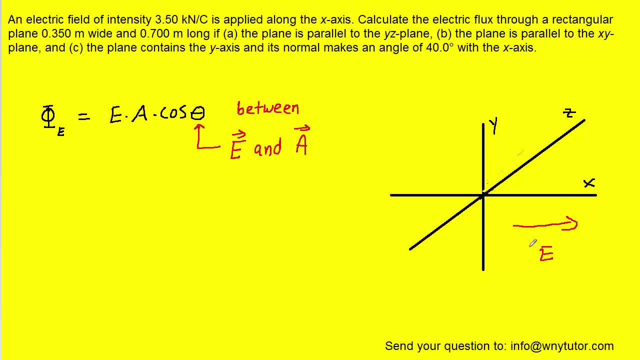 field still pointing along the x direction, But this time the rectangular plane is parallel to the xy plane, And so we're going to attempt to draw a rectangular area that is parallel to the xy plane. Of course, the xy plane is the standard coordinate axes that we're used to using, And if 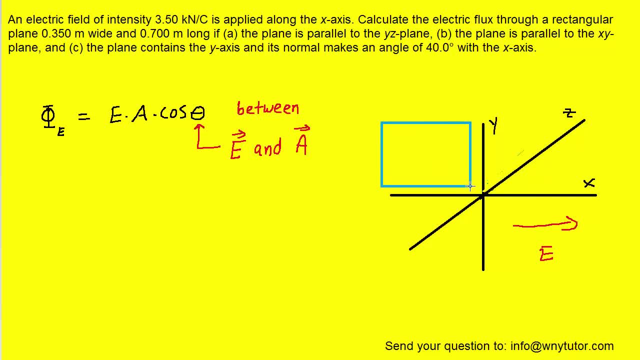 it's parallel to that plane, then that rectangle might look something like this: And remember that we have to draw the area vector for that rectangular plane And, once again, that area vector will always be perpendicular to this rectangular surface And it might be hard to visualize this, but if we draw a line, that's. 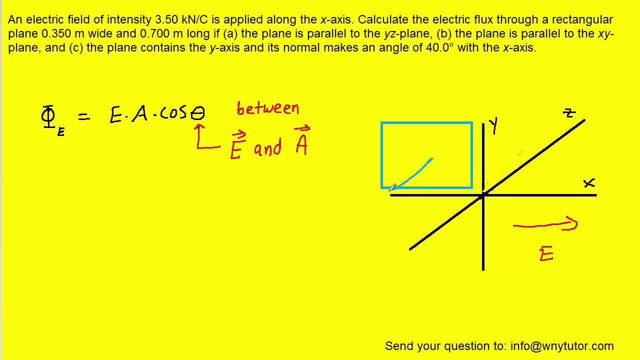 perpendicular, then that line would be projecting along the z axis, That would be our area vector. This would be a 90 degree angle because it's perpendicular with the rectangular plane. And then we have to ask ourselves: what is the angle between that area vector and the electric field? If it helps, you can. 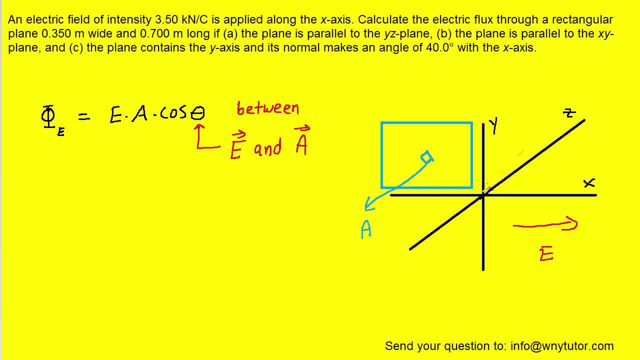 slide this area vector a little bit over and situate it right on the z axis, So that would be an easy way to represent that vector. You can do the same thing with the electric field vector. You can slide it up and put it right on top of the x axis And then hopefully we can see that the angle between